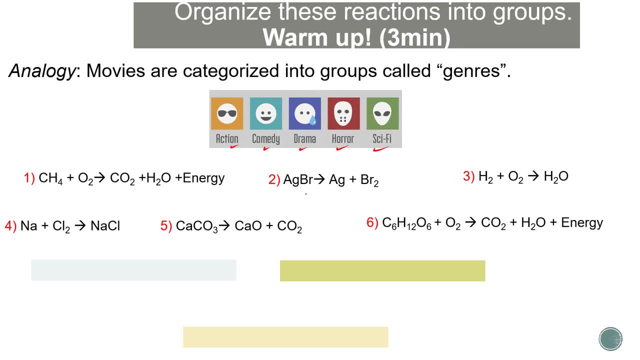 Okay, if I give you, for example, these six chemical reactions, and I asked you to group the ones that look similar with each other, you might think: okay, I'll group reactions one and six. So look at one and look at six. They look similar, right? 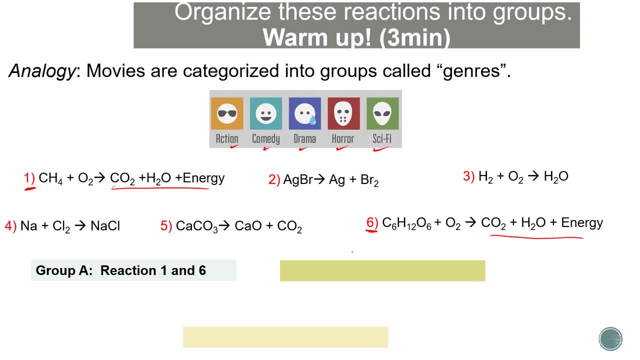 Especially in the product side. Also, group B reactions: three and four. So three and four. they look similar, right? So look product A, LTB, LTBF and so on. And if you were different after classifying chemical reactions: 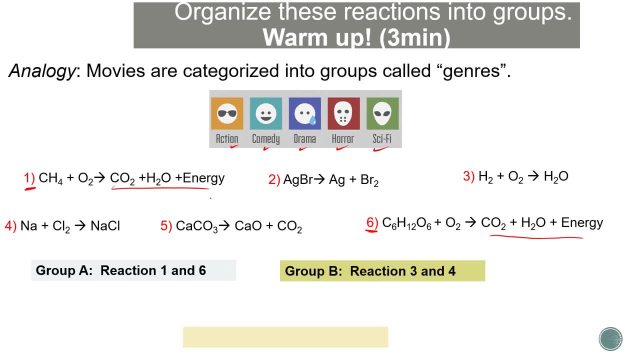 you could add similar make up. We explain this with three and four. For example, if group-B requires three adjustments at a given time, you can group reactions with the открыnt time, for example, and君 back to zero. you can group them with one reaction or three reactions at the other time. Let's say it works very well. 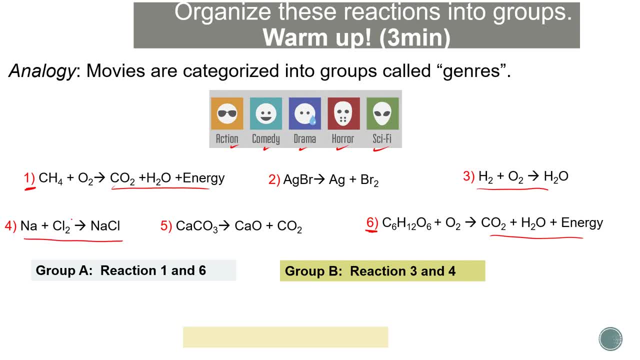 So let's say that group B requires reactions, with all reactions, and君 back to zero. So 3 and 4, they look similar as well. You have 2 reactants, 1 product, 2 reactants, 1 product. 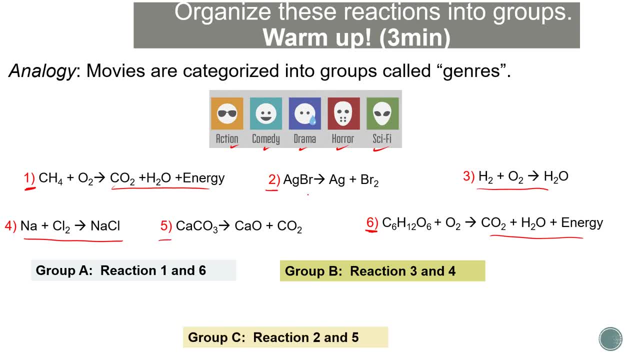 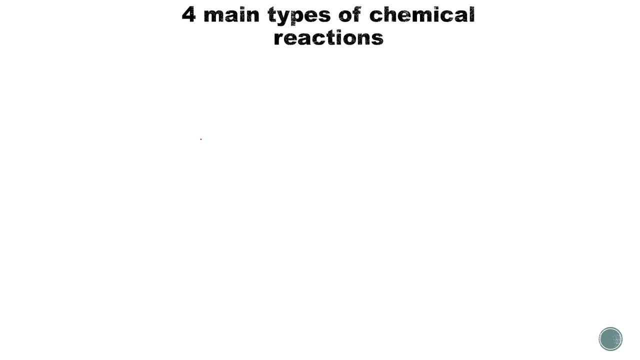 And finally reaction 2 and 5, they also look similar because they have 1 reactant and more than 1 product. So basically we will learn how to classify the types of chemical reactions, okay, So in chemistry in general we have 4 types in general. okay, 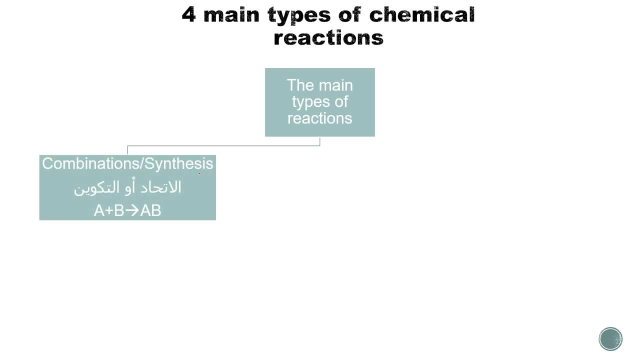 We have combination or synthesis reaction, we have decomposition, we have combustion reaction. combustion means burning- okay. And finally we have replacement reactions, where something will take the place of another thing. okay. For example, A here takes the place of- well, actually this should be B and this should be C- okay. 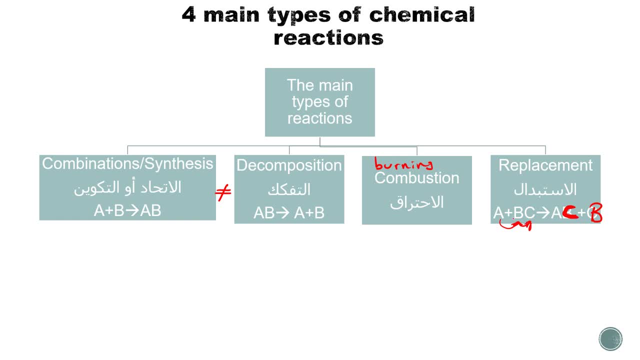 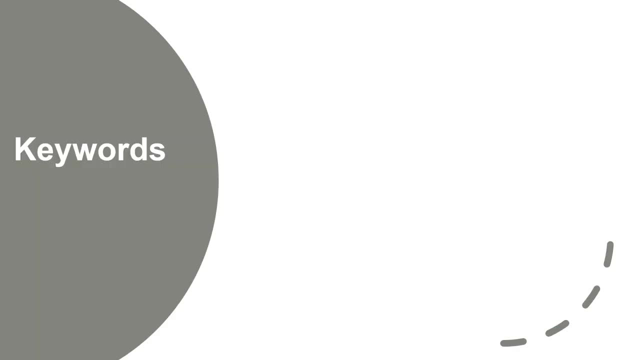 Sorry for that. it has to be like this: okay, A gives me B, C, A plus B, C gives me A, C plus B, And we'll see this in shop, So we'll start with the first one. So these are the keywords, guys. 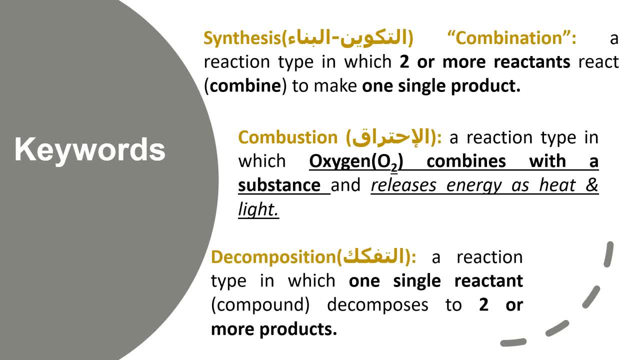 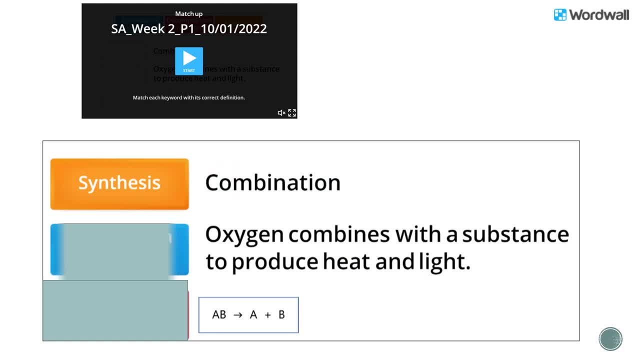 I'll give you some time to read it. You can stop the video. have a look, Let's read it and we will see it, insha'Allah, in the PowerPoint. okay, So, as I told you, chemists distinguish among 4 types of chemical reactions. 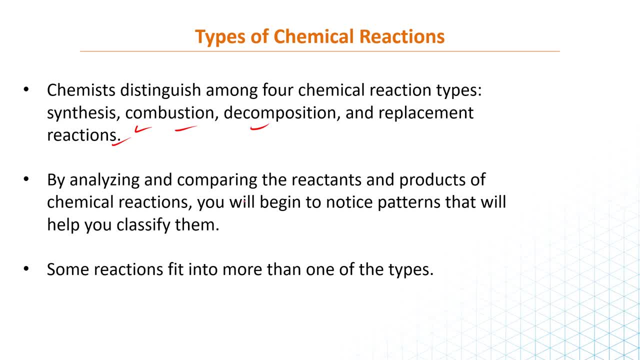 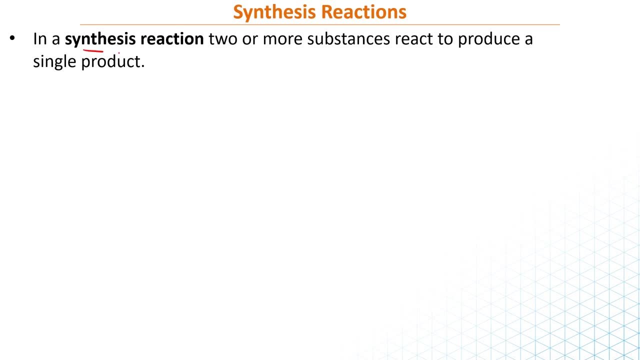 and we can analyze them to notice how they look similar and we can choose one category for each reaction. So let's start with the synthesis reaction. The synthesis reaction is a reaction where two or more substances react to form a single product, So you can have A plus B. 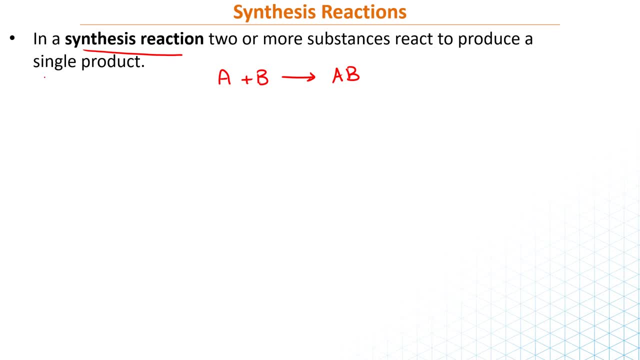 gives me AB Aهم shayy. you have a single product here, يعني يكون عندك ناتج واحد في النواتج. in the product side You can have more reactants, يعني two or more reactants, but only one product. 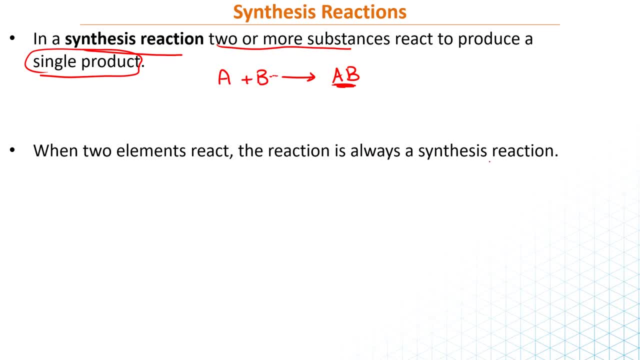 When two elements react, the reaction is always a synthesis reaction. If you have two elements, when they react together, always the reaction is a synthesis reaction, As the example shown below. So look here, guys, You have Na plus Cl2. gives me NaCl. 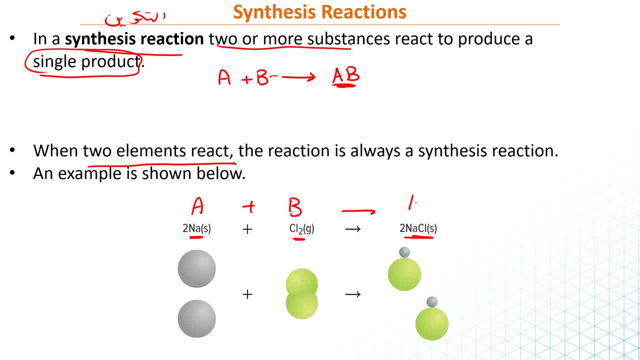 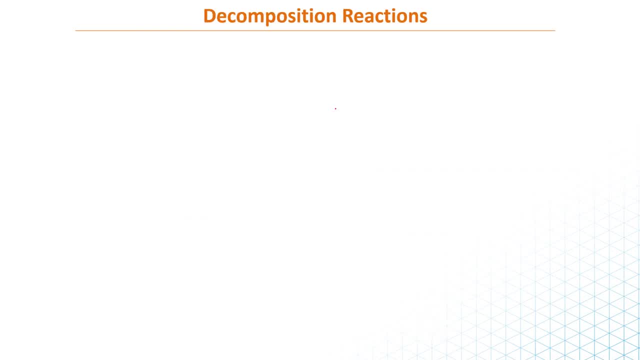 This looks like: A plus B gives me AB. So this is a synthesis reaction, Because you have one product. Now what's the opposite of that? Decomposition reaction? In a decomposition reaction, a single compound breaks down into two or more elements or new compounds. 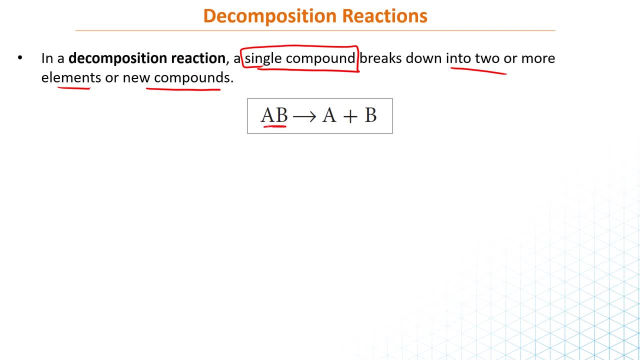 And this is the general formula of it. You have a compound, You have to have a compound So you can have AB gives me A plus B. Or sometimes you can have ABC gives me AB plus C, So the compound can break down and give me a compound and an element. 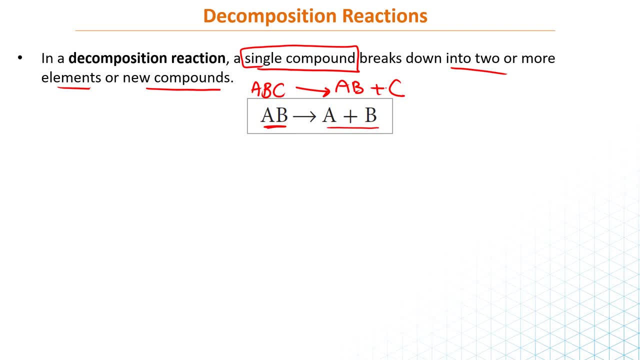 Or it can break down and give me only elements. An example of that is the following: Ammonium nitrate. So this is an ionic compound which we covered in term one. So it will break down into two compounds: Into N2O. 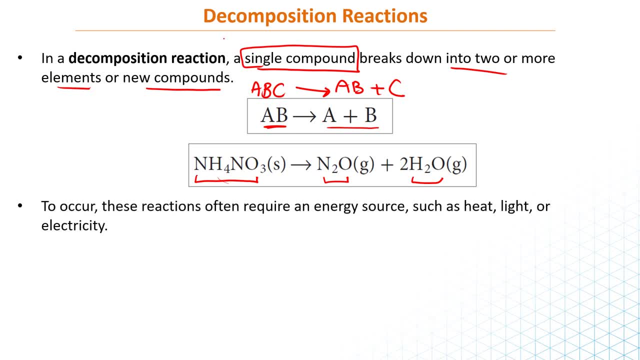 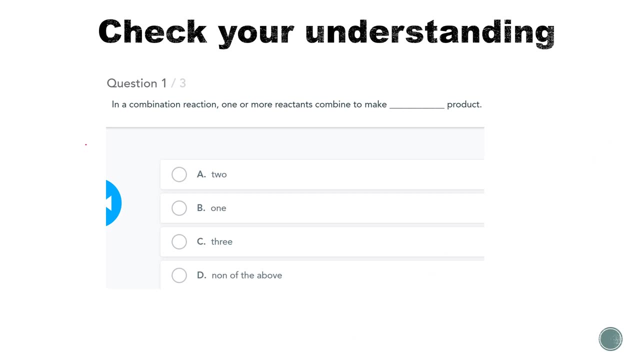 And H2.. So this is a decomposition reaction, Okay, And they often require an energy source to break it down, Like you need to heat it up to break it down, Okay, Or an electricity source, Okay, guys. So try to read this question and try to answer. 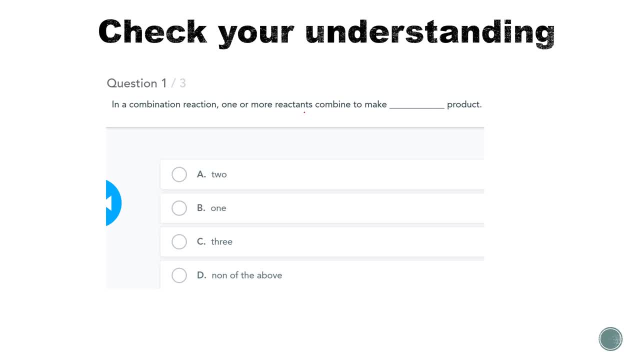 Okay, In a combination reaction one or more reactants combine to make. So combination, guys, is the same as synthesis. So how many products do we make? Remember We make one product, The Of NaCl in water gives Na plus and Cl minus ions. 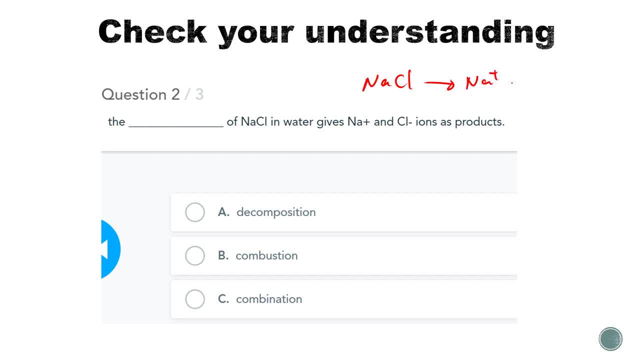 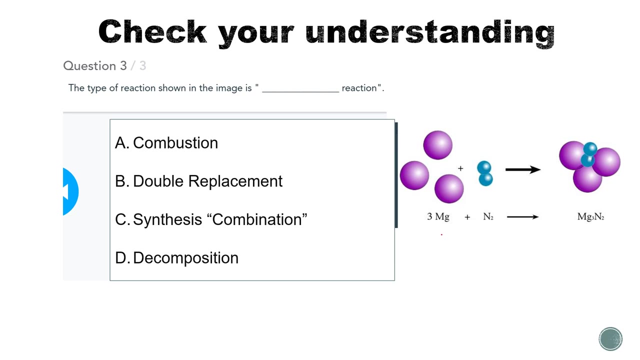 So when you put NaCl in water, it gives you Na plus and Cl minus. So what type of reaction is this? It is decomposition. Okay, Very good. The type of reaction shown in the image is. So have a look here. 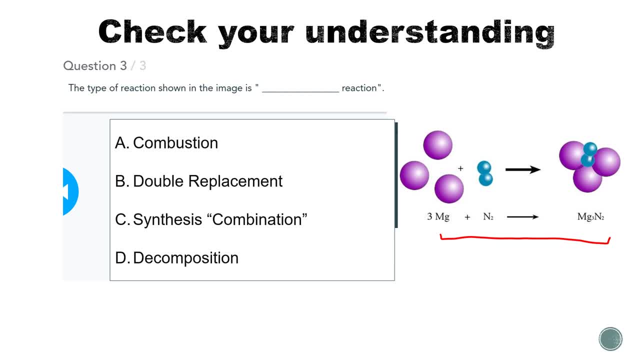 What type of reaction is this, guys? Well done, It's a synthesis reaction, right? Because you have a single product and you have two elements here, Two elements When two elements interact with each other. we said this is always a synthesis reaction. 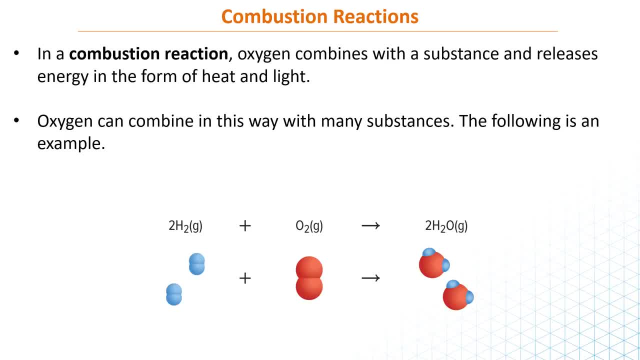 Okay, Now we go to combustion reaction. So we finished synthesis, We finished decomposition. Now let's go and talk about combustion reactions. So in a combustion reaction, oxygen, which is O2, combines with a substance. It combines with a certain substance and releases energy in the form of heat and light. 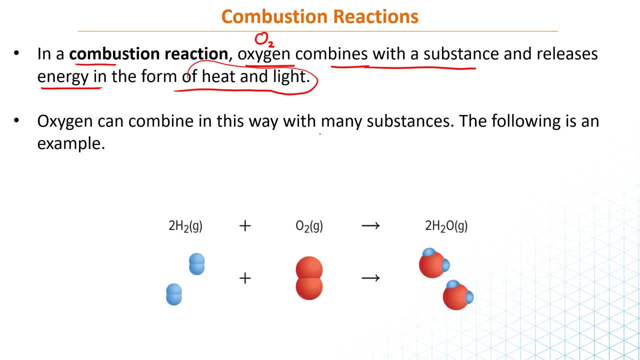 Oxygen can combine in this way with many substances, And this is an example. For example, H2 plus O2 gives me H2, Because we have oxygen here. Okay, then, this is a combustion reaction. You might think: okay, mister, this looks like this. 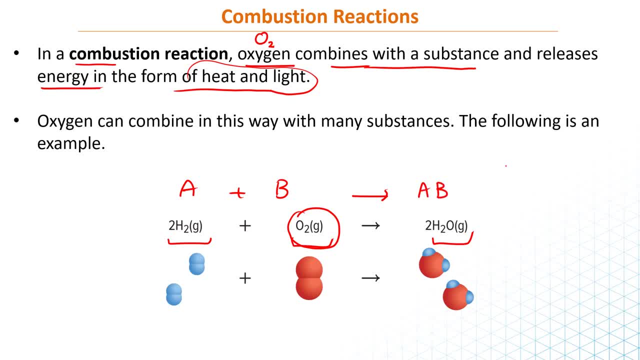 Doesn't it? So this reaction actually is synthesis And also combustion, Because of the oxygen and the heat that you will get. So usually many combustion reactions can be synthesis reactions as well, Okay, and sometimes you can have a hydrocarbon- Okay, CXHY plus O2. 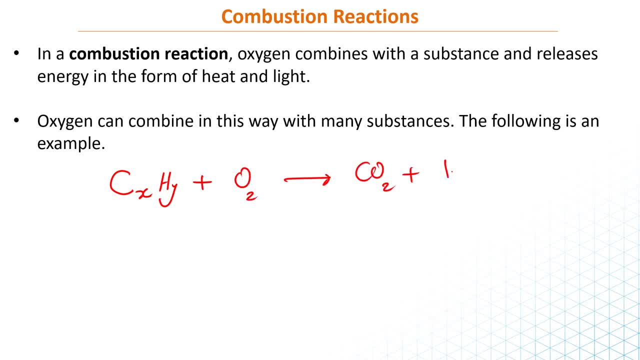 And this will give me CO2 plus H2, Okay, and this will give me CO2 plus H2, And this will give me CO2 plus O2 plus heat. What am I trying to show you here? I'm trying to tell you that if you have any compound that has carbon and hydrogen in it, 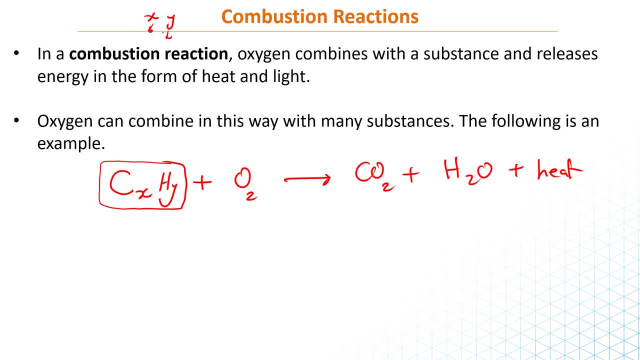 X and Y can be any numbers. Okay, X and Y can be any numbers, And you have oxygen. Then in the products you will get CO2 and H2O And heat, Because this is a combustion reaction. And this is an example, guys, This is methane. This is methane. 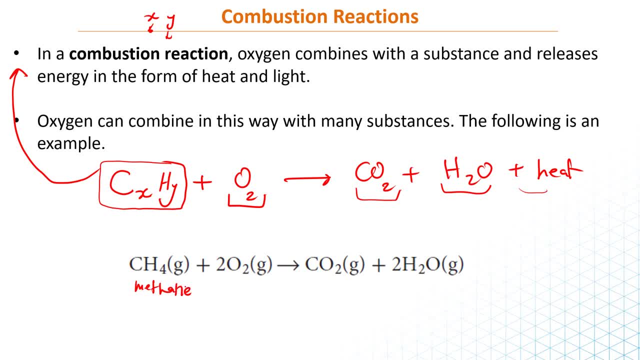 This is a gas. Okay, in the stove, when you try to make fire, This is what happens And you get CO2 and H2O, So this is a combustion reaction. This is not synthesis. Okay, because we have more than one product. In the previous one, we have only one product. 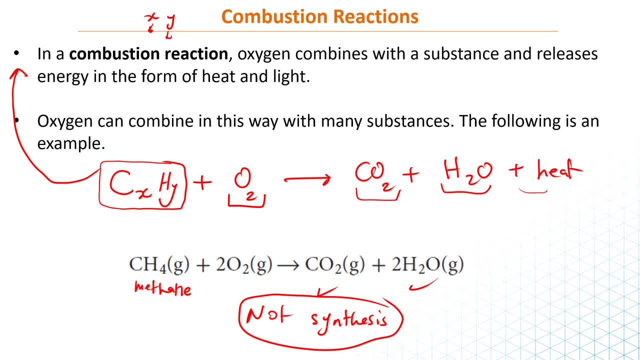 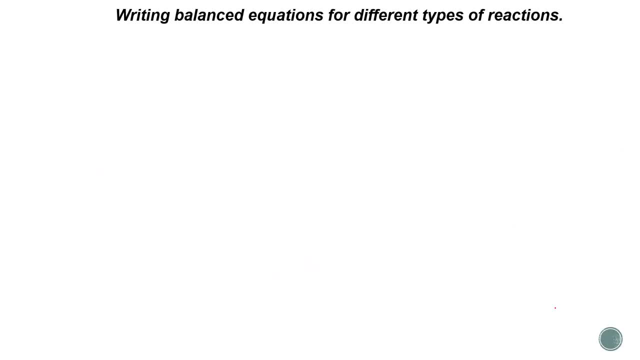 That's why it's synthesis In here. it is not synthesis, okay, Only combustion. So we learned three types of chemical reactions. We learned about synthesis, decomposition and combustion. Now what we are going to do now Is we will write balanced chemical equations For these different types of reactions. 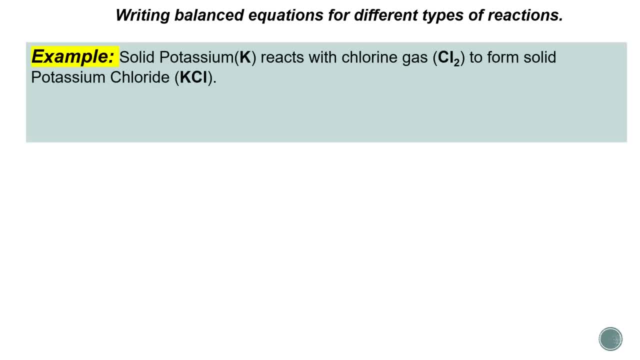 So this is an example. So solid potassium reacts with chlorine gas To form solid potassium Chloride. Write the balanced chemical equation for this reaction. What is the type of this reaction? So now let's write the balanced chemical equation Which we know from the previous lesson. 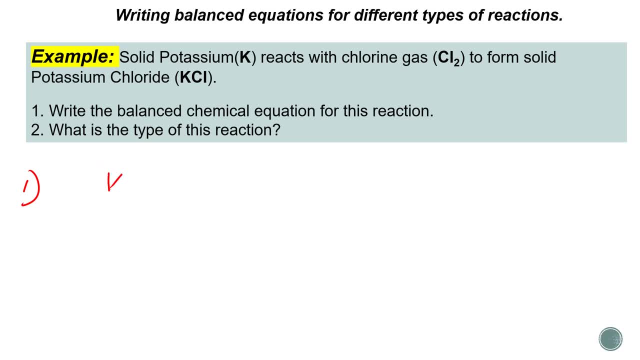 In the previous video we learned how to do it. So K, solid potassium Plus chlorine gas, Cl2 gas Forms, KCl Chloride. Where did I get this from? From here? Is the equation balanced or not? No, here we have 2Cl. 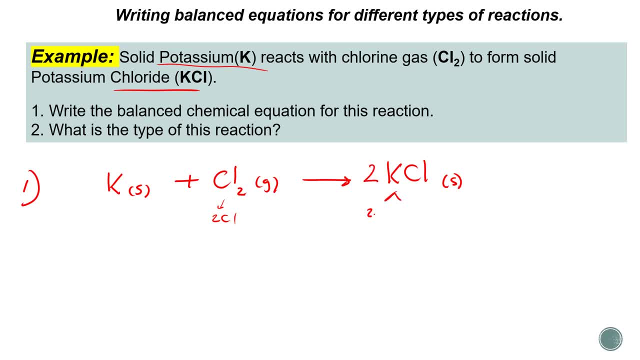 Here we have only one, So let's put 2 here. Now we have 2K and 2Cl, So I need to put 2 here. Now we have the equation balanced. Now our equation is balanced. okay, What is the type of the reaction? 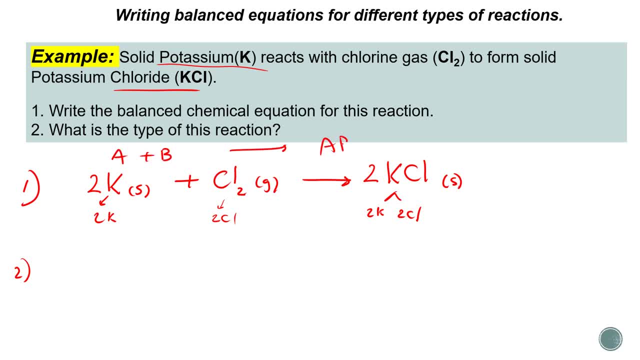 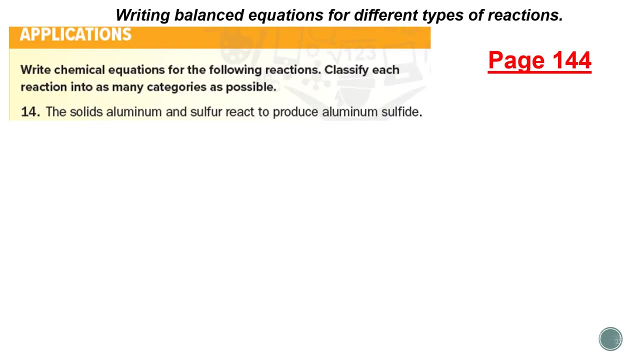 This looks like this right: A plus B gives me AB. Okay, Synthesis. So it is Synthesis, Okay, guys. All right. Now these are some problems. Ignore the page. Maybe you have the page, Maybe you don't have, But this is applications on what we have been talking about. 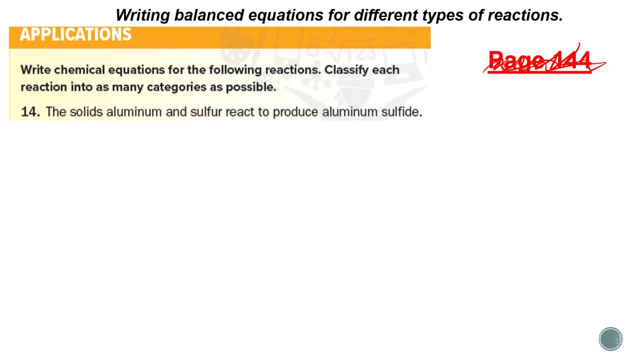 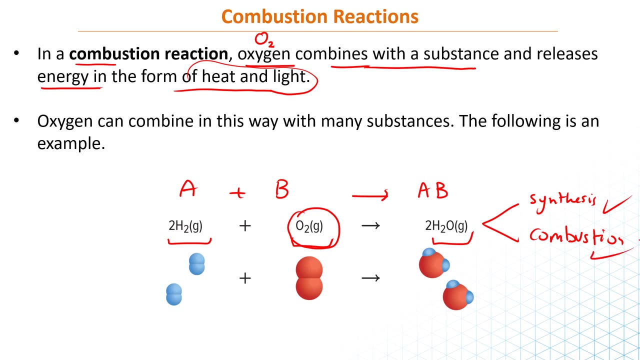 So write a balanced chemical equation for this reaction And classify the reaction Integer Into as many categories as possible. I mean, maybe I have a reaction that has more than one type. How, Like we saw here, This reaction can be synthesis and it also can be combustion. 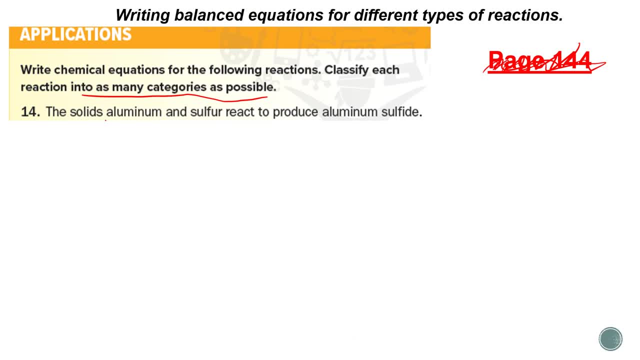 So let's read the question. The solids aluminum and sulfur react to produce aluminum sulfide. Now I told you you need to revise the stuff from term one. Okay, Because they will not give you the formulas sometimes in the exam. So you know that aluminum is Al plus sulfur is S. 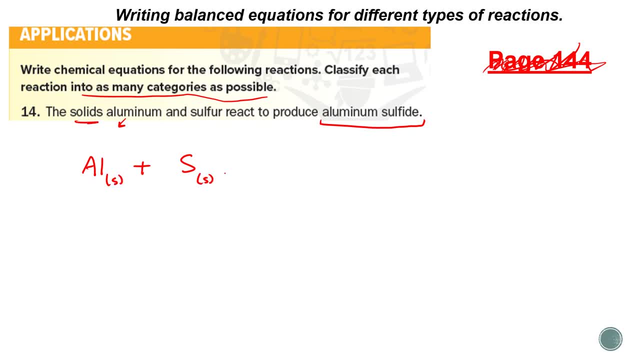 Solids or galaxy solids, So they should be solids. Gives me aluminum. sulfide is an ionic compound. Okay, And the periodic table is in the exam In the questions. I mean we can use it in certain questions. Let's go to the question. 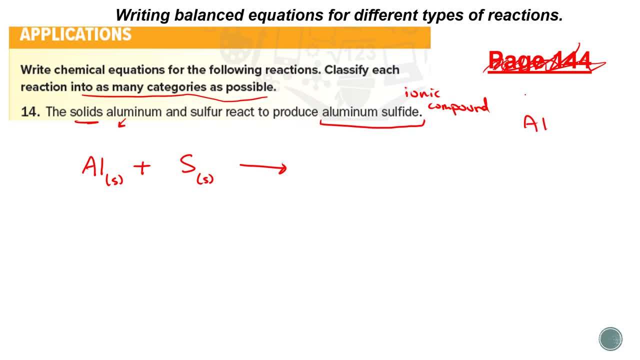 And we take the information from the periodic table. So Al is in group 13, Sulfide is in group 16, So the charge here is plus 3, Charge here is minus 2. Remember term one. Exchange the charges And this will be Al2S3. 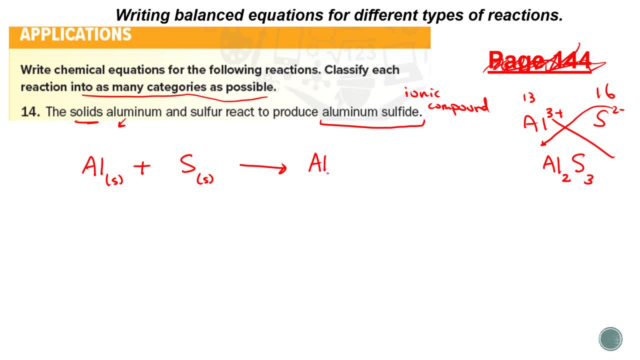 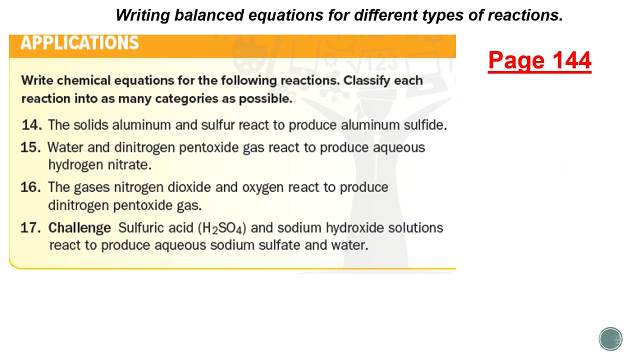 So aluminum sulfide is Al2S3. Now balance the equation 2Al here, so put 2. You have 3S, so put 3. What type of reaction is this Synthesis? Okay, guys, Alright. So these are some problems that you have in your book. 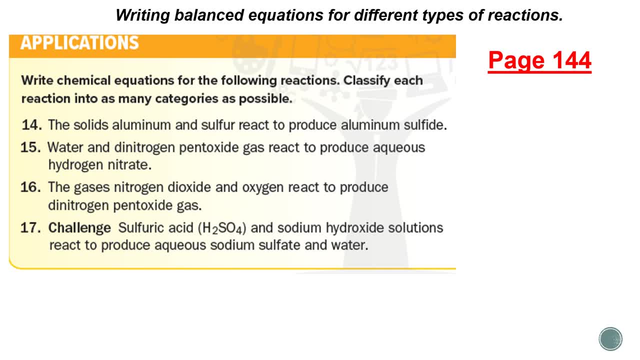 You can try them on your own And you will find the solutions down here. Okay, This last one, This last one here. we'll see later, inshallah. Okay, It's a replacement reaction. We haven't studied it yet, Replacement reaction, Which is the challenge. 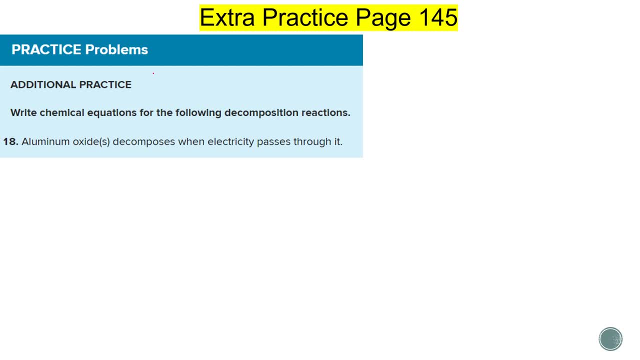 Okay, We'll see it later, inshallah. Okay, Write chemical equations for the following decomposition reactions: So they are very kind here. They told you it's already a decomposition reaction. So aluminum oxide decomposes. It means it decomposes When electricity passes through it. 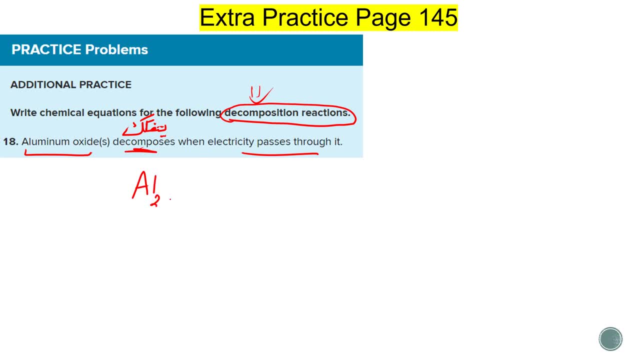 Now Aluminum oxide is Al2O3, Because Al charges have positive 3 And the oxygen is negative 2. Exchange: We have Al2O3. So Al2O3 decomposes. They did not tell you What are the products, But this compound decomposes. It means it gives me its elements, right. 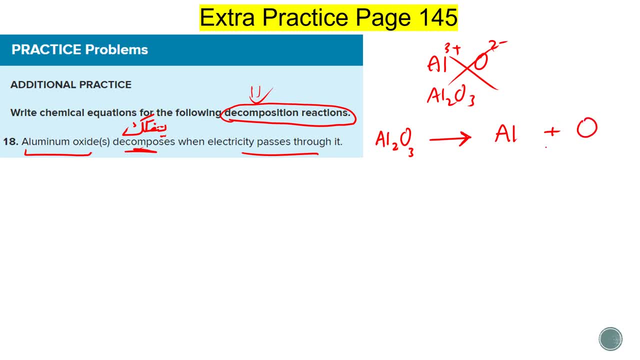 So Al plus O. But I told you guys, I told you Oxygen alone, We have to put 2 for it Because it's a diatomic molecule. So O2 Balance the equation. You have 3 here, You have 2 here, So I'll put 3. 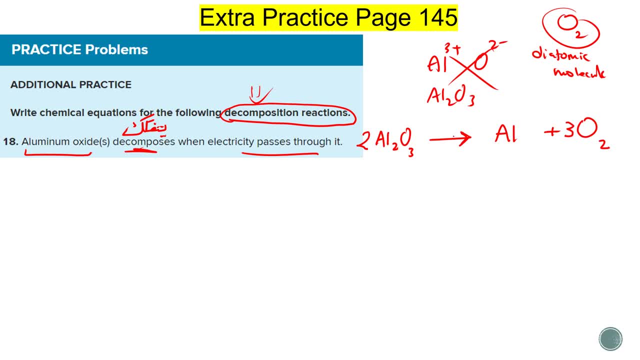 And I will put. I will put 2, And here I will put 4, Because now I have 4 Al And I have 6 oxygens, And here I have 4 Al And 6 oxygens. Okay, So this is very important. Now You can try these questions on your own. 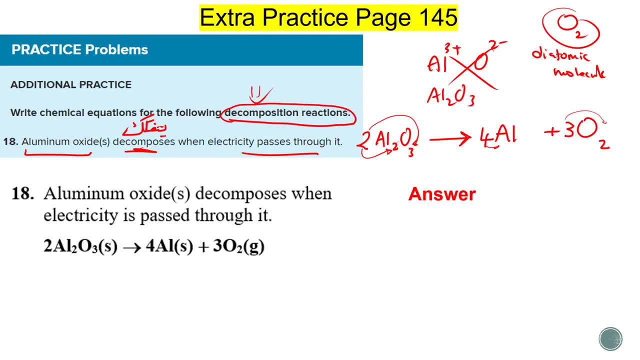 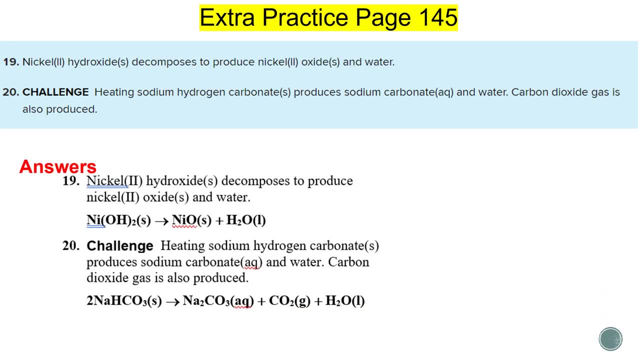 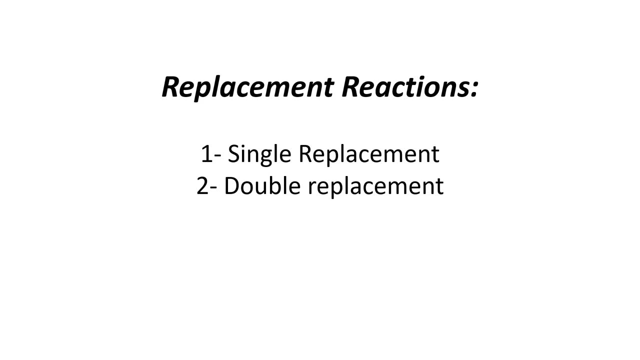 Okay, This is a continuation. Decomposition reactions: You can try them on your own. Stop the video now And the solutions are here. Okay, All right, And that's the end of the first 3 types Of Of the 4 types of chemical reactions. Okay, So now we'll go to the 4th type. 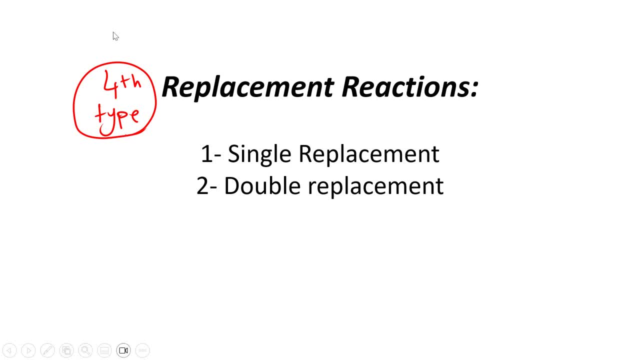 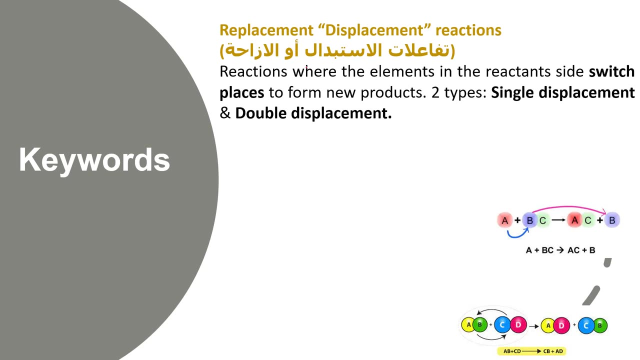 Replacement reactions, guys. Okay, Now we'll talk about replacement reactions. So we have 2 types of replacement reactions. We have single replacement And we have double replacement. So what is a single? What are replacement reactions in general? Replacement reactions, Reactions of replacement reactions. 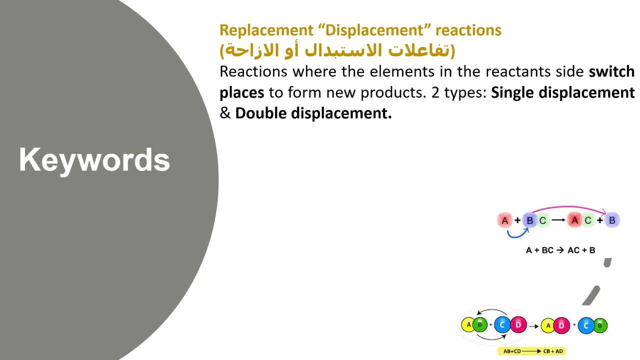 There is a replacement with me. It happens. There are reactions where the elements In the reactant side Switch places To form new products. We have single and Double. So single replacement reaction Is a reaction in which the atoms Of one element replaces the atoms Of another element in a compound. 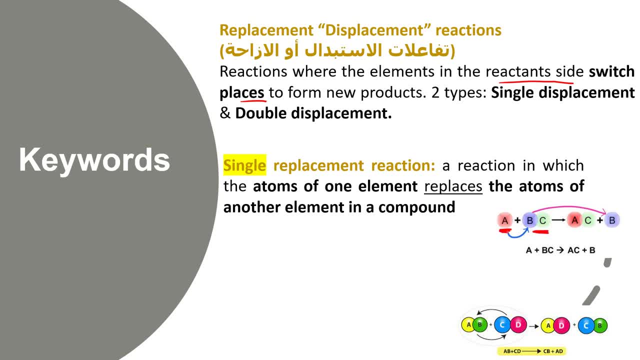 So you have an element And you have a compound. Look A here Took the place of B And removed it right, So it's called a single replacement reaction. Now, If you have 2 compounds And each one, Each element in the compound, switches Places. 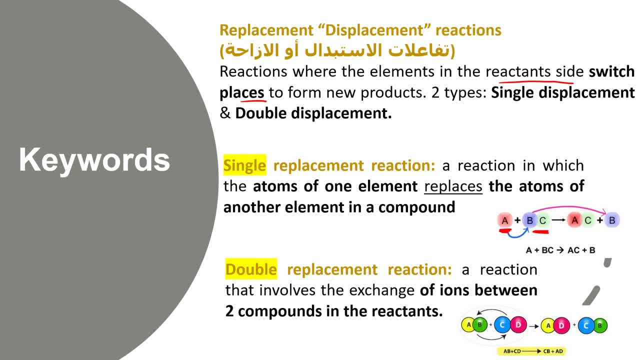 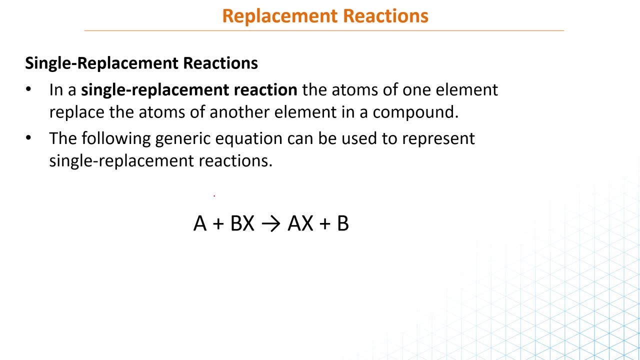 Like AB and CD. Look here: B went And C And D came to A To A. yes, So this is called a double replacement reaction. So this is the general formula Of single replacement reactions, guys. A plus BX gives me AX plus B. So A takes the place of B. 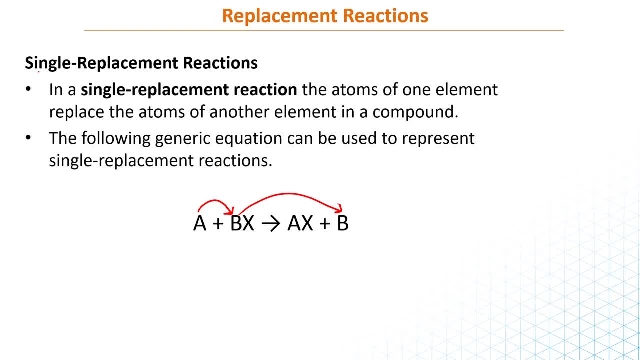 And B goes here. This is what we mean by single replacement reactions. But we have a problem here. How can we know If A will be able to replace B? I mean, who is stronger? I mean, for example- You can think about this, For example: 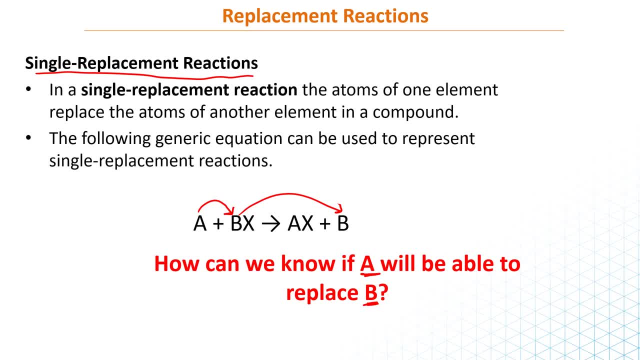 You and your sister or your brother. Your brother is older. You have, for example, You have 2 siblings. You have 2 siblings, yes, Brother and sister, Or brother and sister. One is older than you, One is younger than you, And you guys are sitting, Want to sit in the front seat of the car? 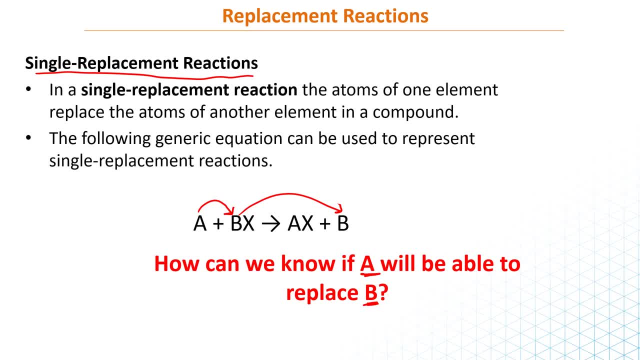 You want to sit in the front seat of the car. Now, if the older brother is sitting, You are weaker than him or her right, So you cannot remove them. But if the younger brother is sitting, You have more power than them, So you can remove them. 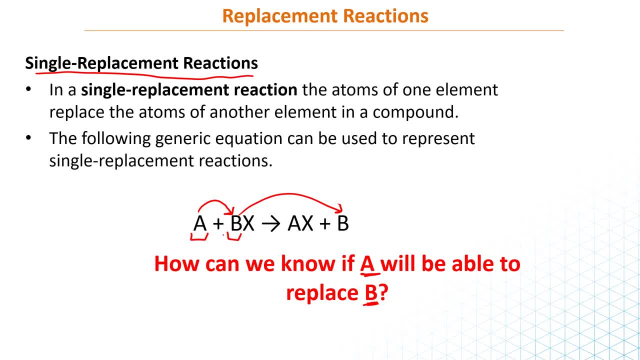 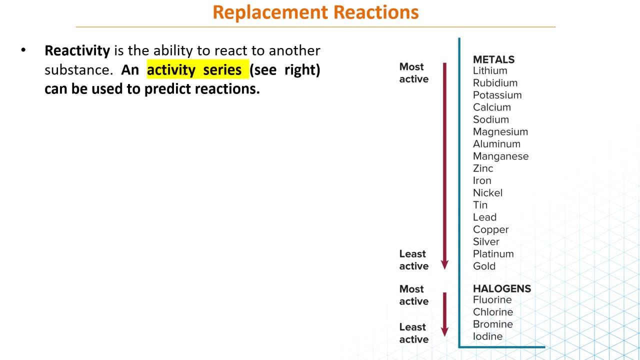 So same thing. here We have to compare between the power of A and B. Will A be able to remove B or not For the reaction to happen? Okay, How can we know that We use something called The reactivity series? Okay, So the reactivity is the ability to react to another substance. 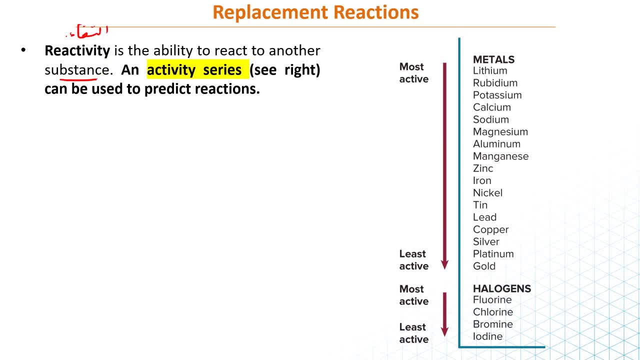 Reactivity is the reactivity. What is reactivity? I mean? how many? I mean- how can I say this in Arabic? The ability to react. So the ability Or the ability to react Is the ability to react with another substance And an activity series. 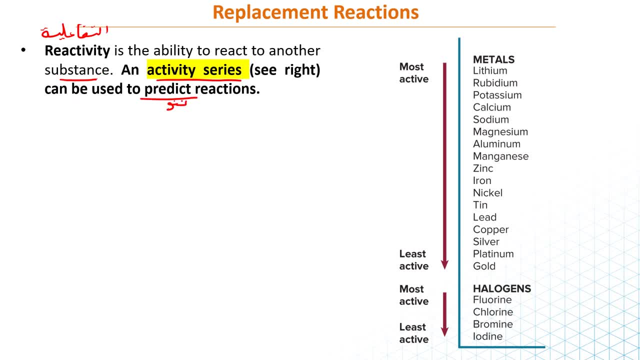 Can be used to predict, To predict The reactions. So we have two sides. This is the activity series, guys Activity Series. So This side here is for metals. So up here metals, Down here halogens, F, Cl, Br, I, And here the metals. 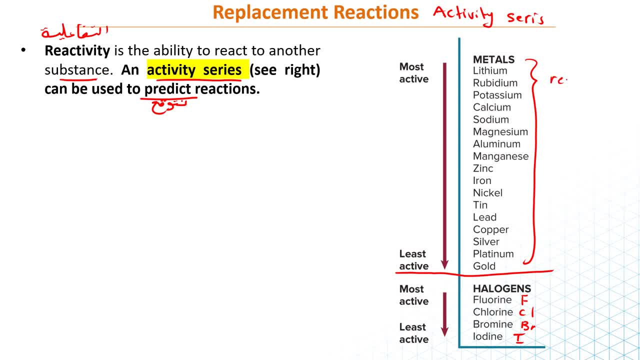 So these Replace Each other And these Replace Each other. Up here, The most active, The strongest, The least active, The weakest. So A metal Will not always replace another metal In a compound dissolved in water, Because of different reactivities, And halogens frequently replace other halogens in reactions. 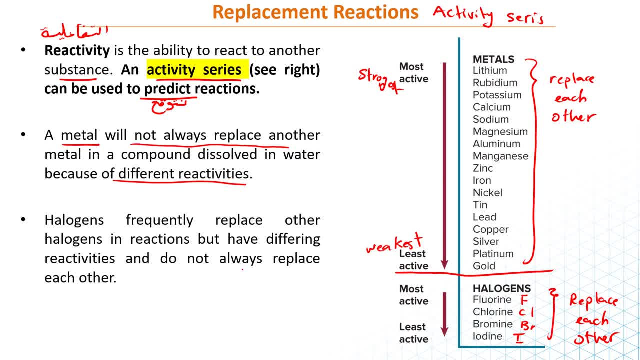 But have different reactivities And do not always replace each other. For example, Imagine you have F Plus A Cl. Now these will replace each other. Now we have F And we have Cl. Can F remove Cl or not? Who is stronger? F is stronger than Cl. 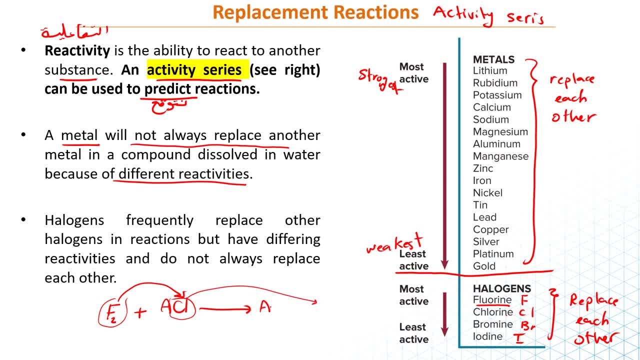 So it will be able to remove it. So now we will have Af Plus Cl2. This is Sodium And this is Zinc. So imagine you have Zinc Plus NaB. Now will the Zn be able to remove Na or not? Zn is weaker than Na because it is below it. 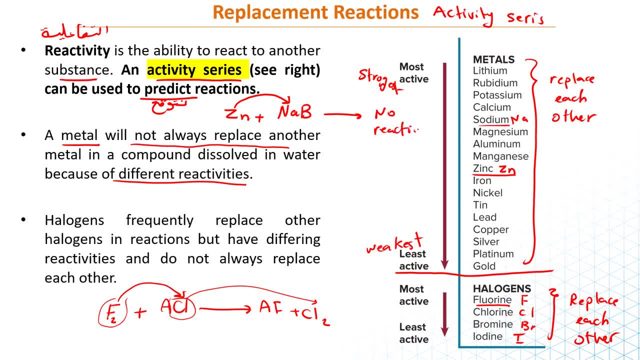 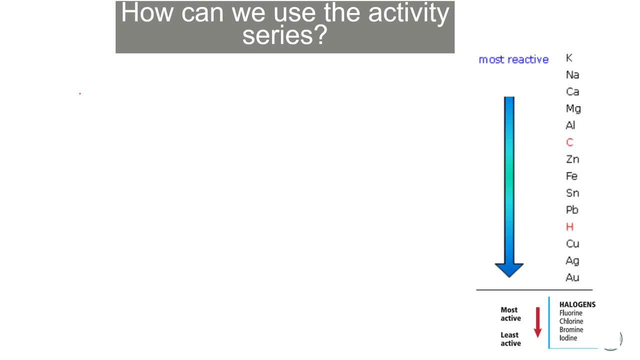 So no reaction. You will not be able to. So you will have the same thing: Zn plus NaB. This is how we use the activity series To predict these reactions. Okay, So, for example, Imagine I have Mg Plus CuCl And they will tell you. 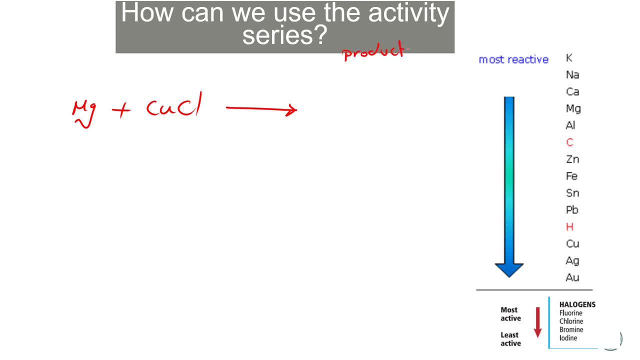 What is the product? So they will ask you: What is the product? So from here We have to know that this is an element And this is a component, Right? So this is an element And this is a compound. So whenever you see something like this, 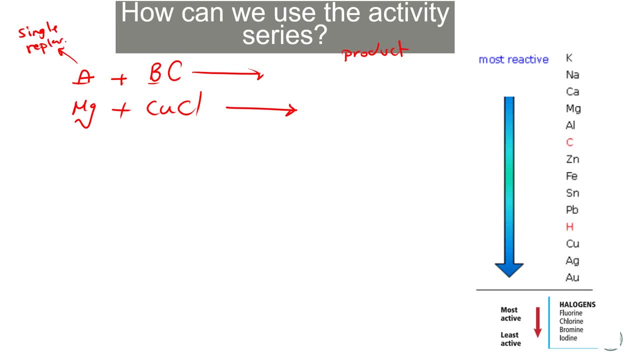 An element and a component. Think about single replacement. And when you think about single replacement, You know you will use the activity series. It will give you in the exam What we have to memorize it. It will come in the exam But we have to know how to use it. 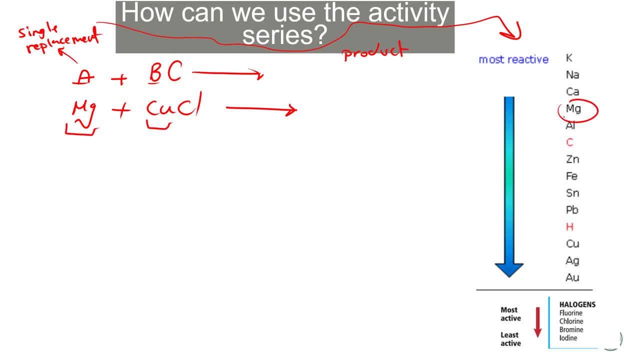 So we need to know if this will happen or not. Mg is stronger than Cu, so it will remove it. Okay, so we are going to have MgCl2 plus Cu. Now what about Au plus AgCl? Can Au remove Ag? 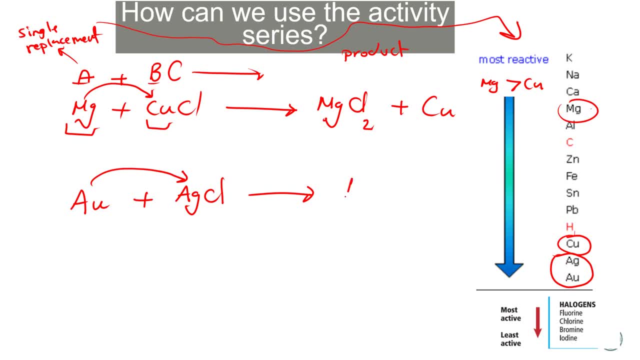 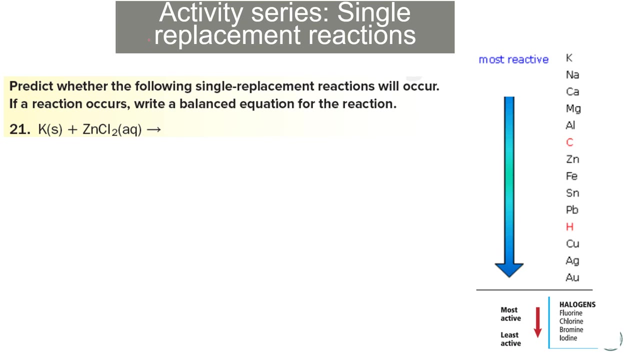 Au is weaker than Ag, so it's weaker, So no reaction. This is how we use the activity series. Okay, So this is the type of the question that you have in your book: Predict Whether the following single replacement reactions will occur. 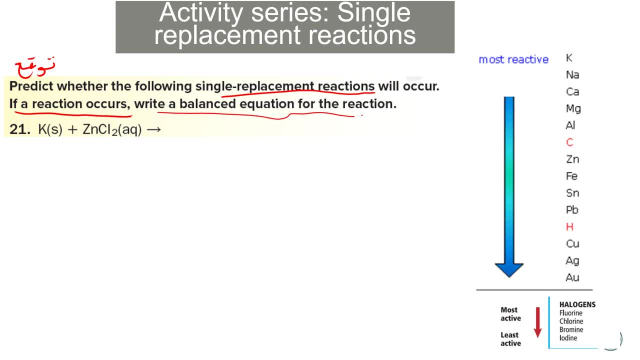 If a reaction occurs, write a balanced equation for the reaction, So K plus ZnCl2.. So you go to the activity series, find K. K is stronger than 1, and Zn is below here right. So K plus ZnCl2 gives me. 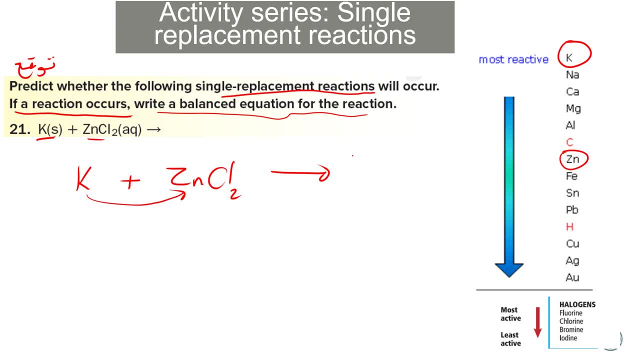 Can the K remove Zn? Yes, because it's stronger. So K plus KCl plus Zn. Let's balance the equation. We have 2Cl here, so put 2 here. Now we have 2K, so put 2 here. 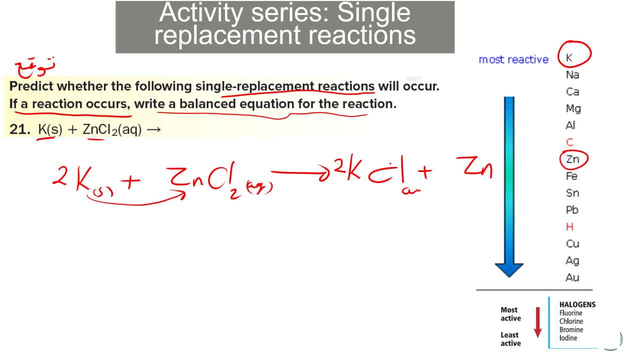 Solid, Aq, Aq and solid. Okay, The minerals are solid because Zn is a metal. These are metals. Okay, This is Zn plus 2, because Zn has a charge of plus 2.. Cl has a charge of minus 1.. 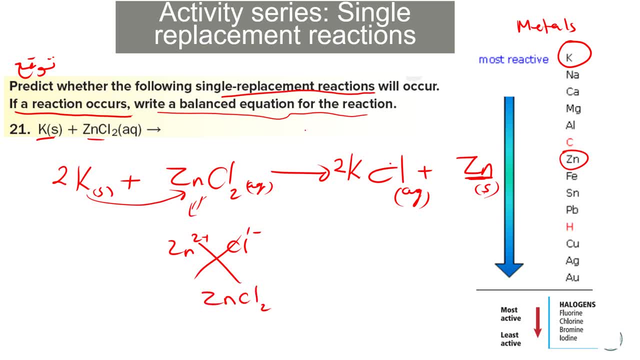 We exchange, Then you get ZnCl2.. KCl because K is present in group 1.. The study break is additional, So K plus 1.. Cl minus 1. Exchange KCl. That's why I told you it's very important to revise this stuff from term 1,, guys. 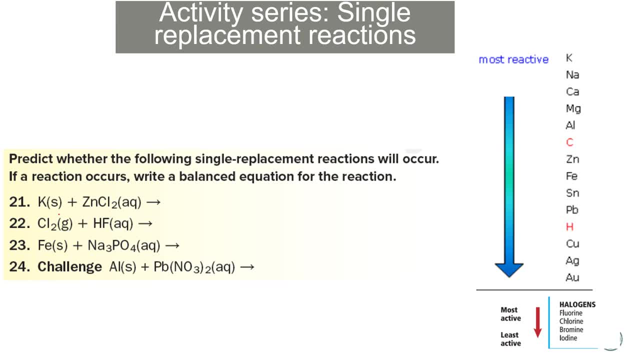 Okay, So let's do 22.. So Cl2 and Hn. So here you have down here F, Cl, Br and I. So now we look at Cl and we look at F. So the replacement will not happen between Cl and H, because H is present above here. 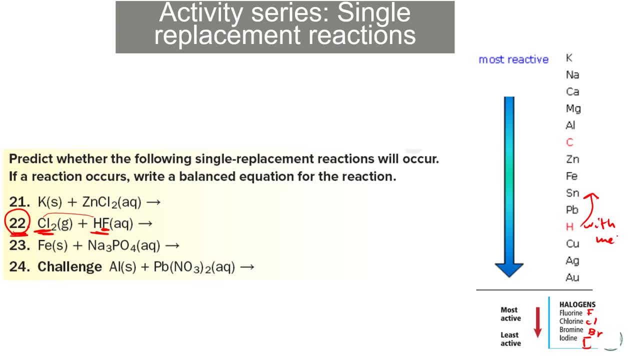 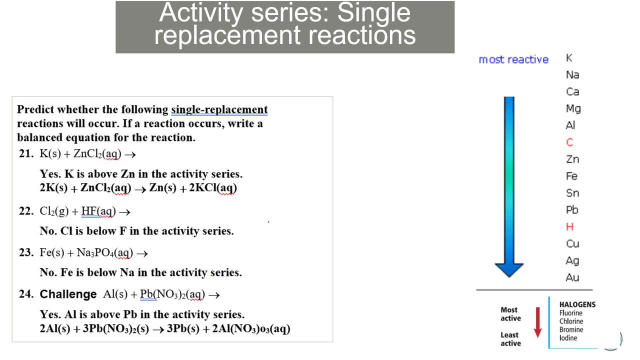 Okay, H with metals, These 4 are with each other. They are what happens between them. Cl is weaker than F because it's under it, So No reaction. Okay, These are the answers to these questions, guys, So you can try them on your own and check the solutions here. 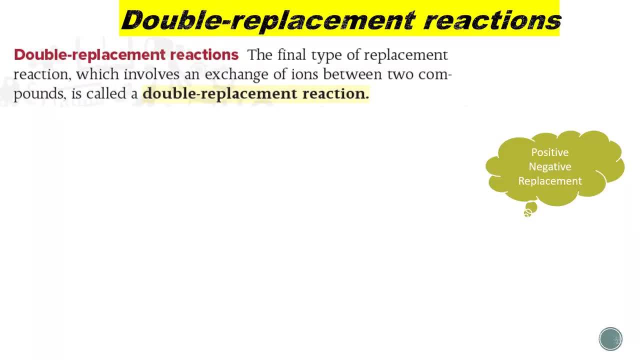 And that's the end of single replacement reactions. So now we go to the last part, which is double replacement reactions. So double replacement reactions is the final type And involves an exchange. So double replacement reactions is an exchange of ions between two compounds. 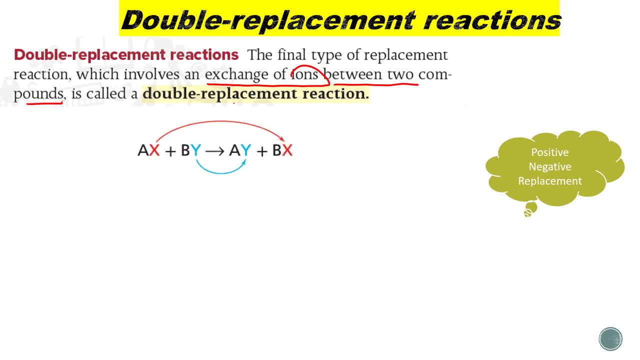 So look here: What do we mean by exchange of ions? Usually these two compounds are ionic compounds. What do we mean? We mean that you have A+ and X- and here you have B+ and Y- Yes, So how do you get a double replacement? 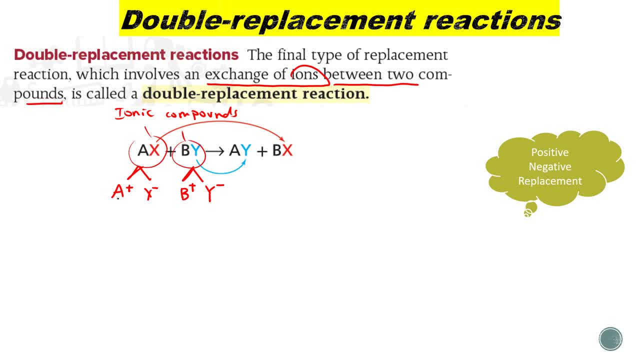 A double replacement happens when the ionic compounds from this compound go with the negative one from this compound, So A and Y, can you see? And the ionic compounds from this compound go with the negative one from this compound, So B and X. 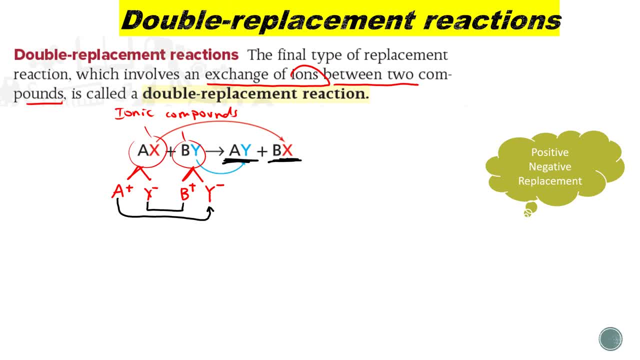 Switch, double switch Because we have two switches. that's why we call double replacement reaction. And this is an example. guys, These are all compounds that we saw in the first study section. Many of them are ionic compounds, many of them are acids and so on. 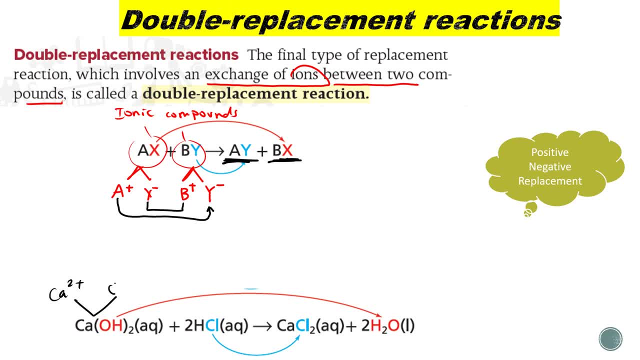 For example, here you have Ca+ and OH- and here you have H+ and Cl- So what will happen is that the H+ will go with the OH- and the Ca+ will go with the Cl- So Ca+ and Cl- we have this. 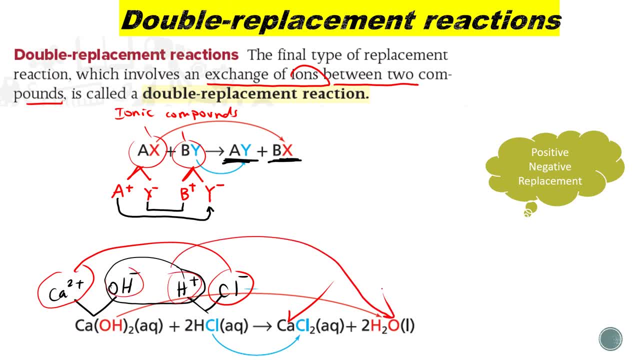 H+ and OH- gives me water. We will learn, inshallah, about this kind of reactions in the next lessons as well. We will have more, a lot of practice on it. Okay, Because we will see it a lot. 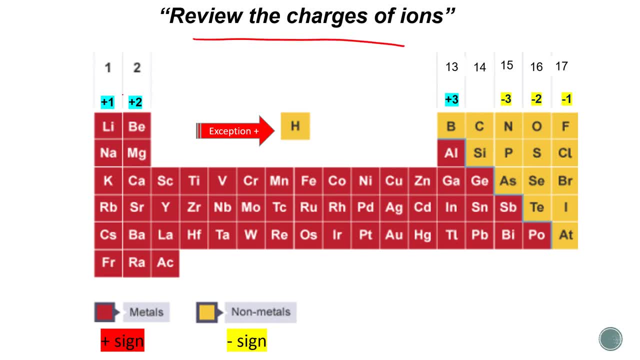 So this is just for you to remember the charges guys Remember in group 1, what their charges are In group 2, what their charges are 13,, 15,, 16,, 17.. This is from term 1.. 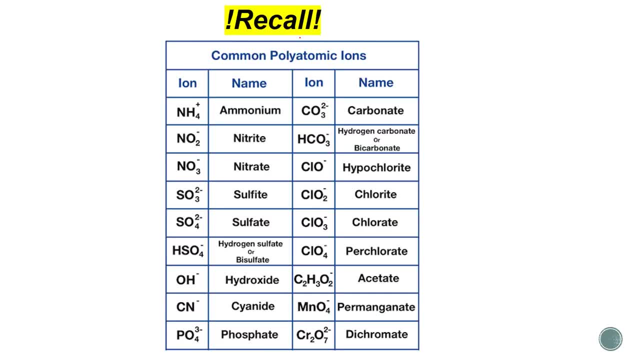 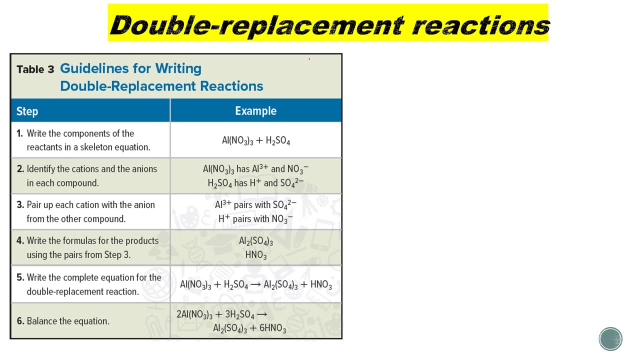 Remember, Remember, Very important- And you should remember the polyatomic ions from term 1.. You should remember these things, guys. Okay, Because you already studied it. So how do we write double replacement reactions, Okay? Okay, Meaning you have Al, NO3,, 3, plus H2.. 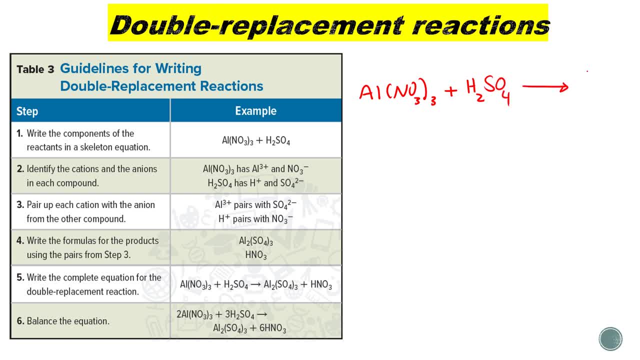 SO4.. What is the product? What we want to do is we want to know what the product is. Okay, So how do we do this? First of all, when we have two compounds. when we have two compounds and you notice that these are ionic compounds, 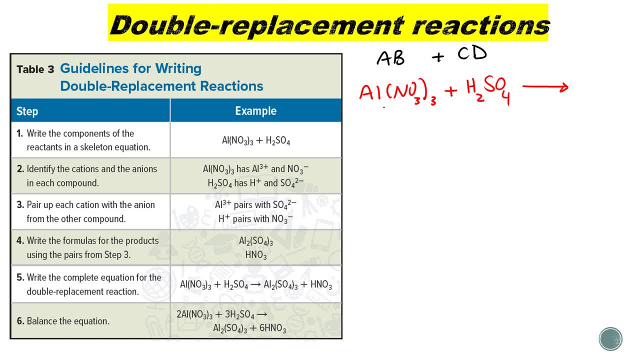 so ionic compounds- and this is an acid- always break down these two into their ions. So what are the ions here? Al plus 3, and NO3, minus. How did we know these things From the first term? 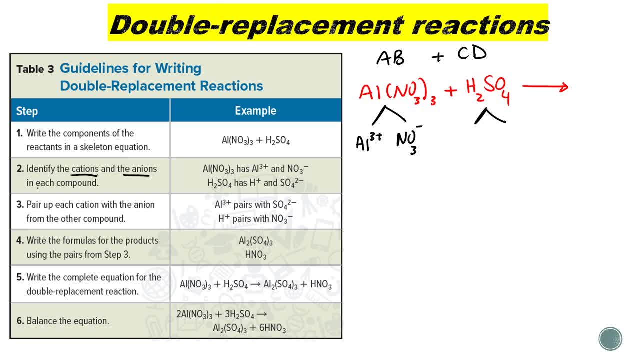 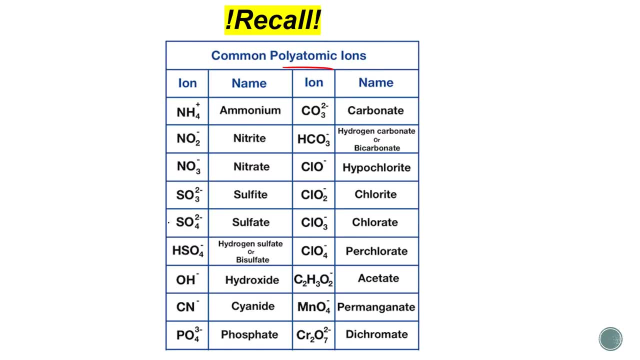 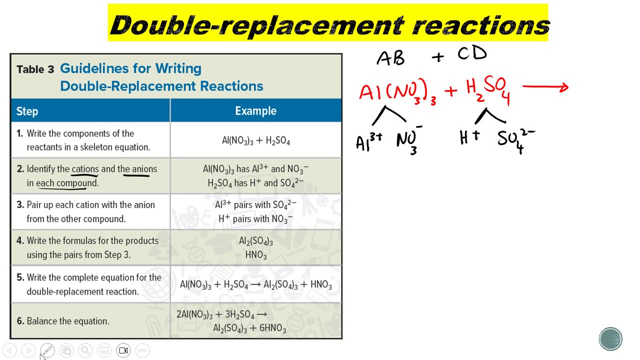 This is a compound, So identify the cations and the anions in each compound. Okay, It's H+- SO4, minus 2.. Here's SO4, minus 2.. Here's NO3, minus 1.. After that, what you need to do, 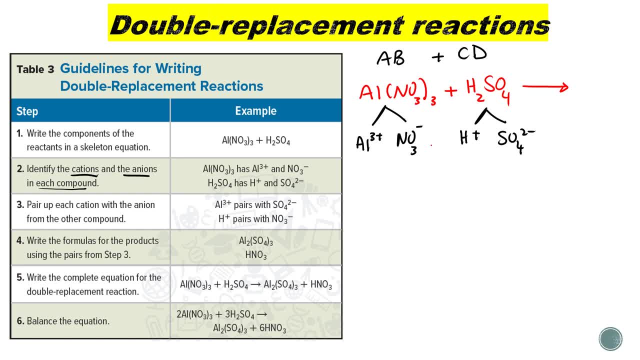 you need to make a compound between the positive and the negative ions in each side. So take Al with SO4, and H+ with NO3, minus So, Al plus 3, and SO4, minus 2.. 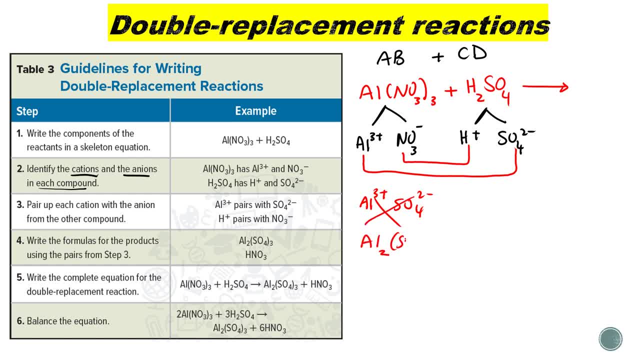 The compound that they will make is Al2SO4, 3.. And the compound between H+ and NO3, minus will be 1 nitric acid, Okay, HNO3.. So basically, your product is going to be. 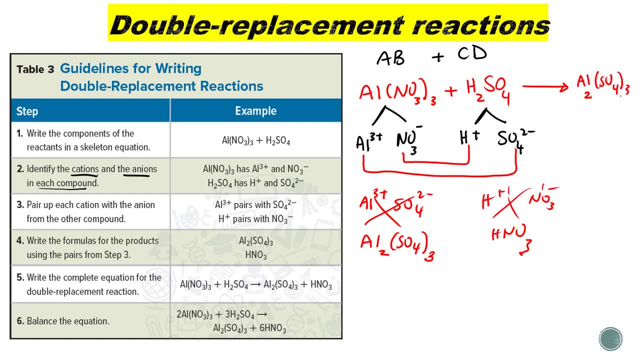 Al2SO4, 3, plus HNO3.. So this is what they told you here. Pair this with this and this with this, And now you have the two compounds- and write them in the products. Did we finish? 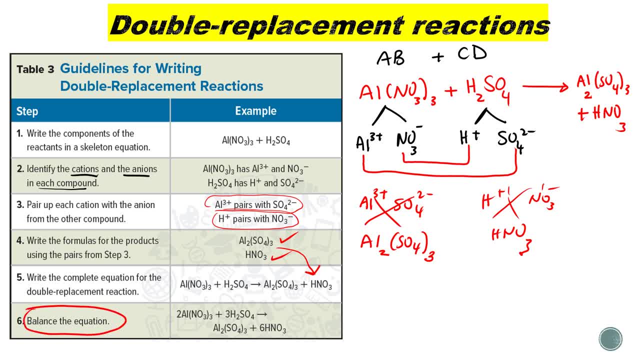 No, The last thing that you need to do is to balance the equation. What? What did we learn in the first lesson? Okay, How can we balance this equation? guys? Look here: NO3, here NO3.. We have 3 of NO3, right? 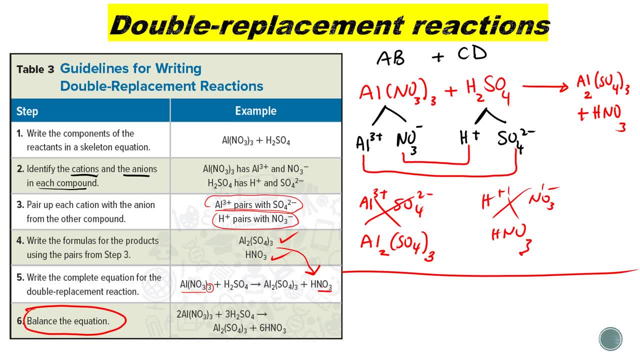 And here we have only 1.. Don't worry about it. First of all, worry about the elements. Here we have 2Al, So write 2. here Now we have 6NO3.. Right, And here we have 1O3.. 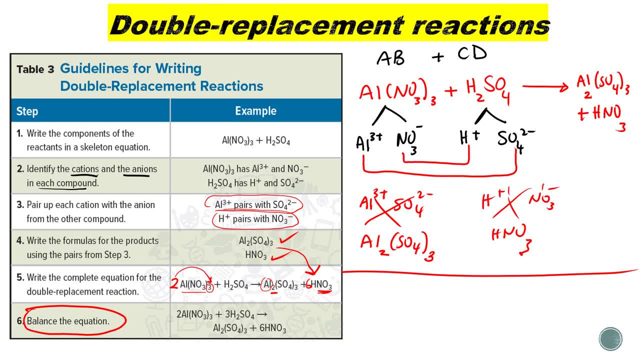 So we need to write 6 here, Alright, And here we have 3SO4. And here we have only 1SO4. So we need to write 3 here, And this is how we balance the equation, guys. 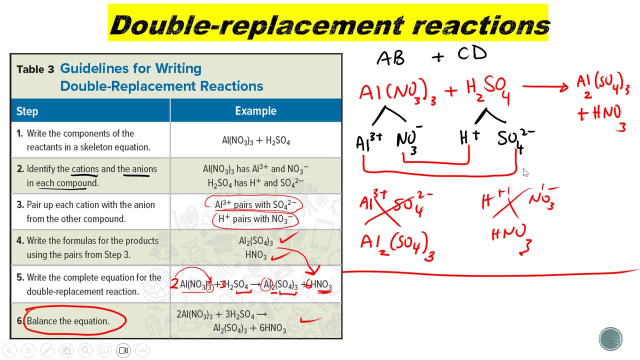 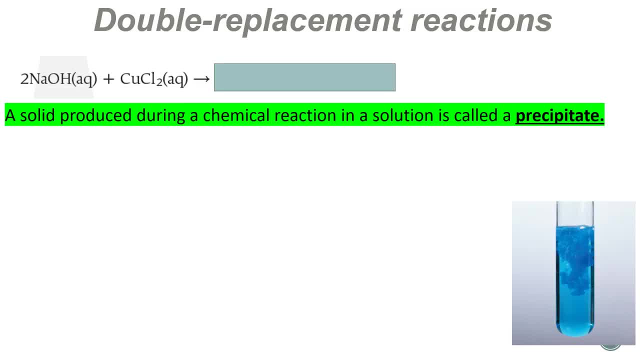 Okay, This is the first lesson, So you can also practice on balancing these types of equations. So you can also practice on balancing these types of equations. So you can also practice on balancing these types of equations. Okay, Double replacement reactions. 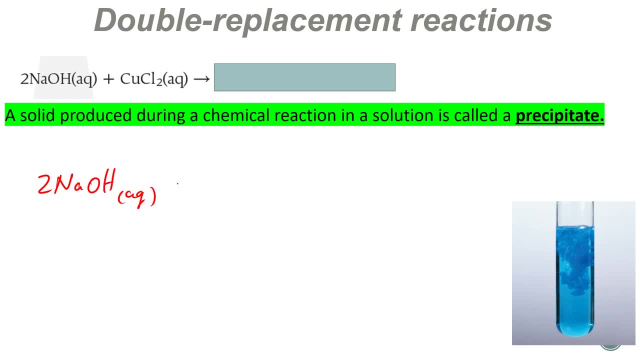 For example, Imagine they give you this reaction: NAOH Aq plus CuCO2, Aq. NAOH Aq plus CuCO2, Aq NAOH Aq plus CuCO2, Aq. 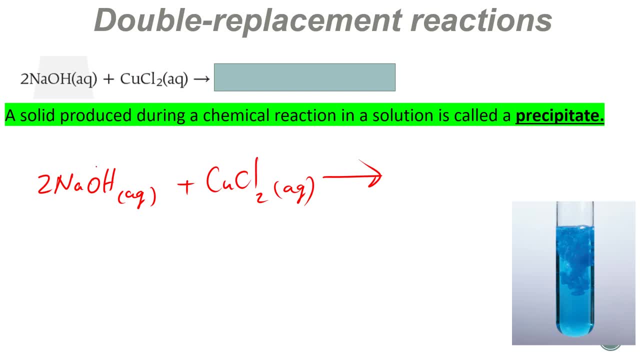 And they want the product. When we see something like this, we need to think about double replacement reactions. When we see something like this, we need to think about double replacement reactions. So now the ions: here Na plus, OH minus, and here Cu plus 2 and Cl minus 1. 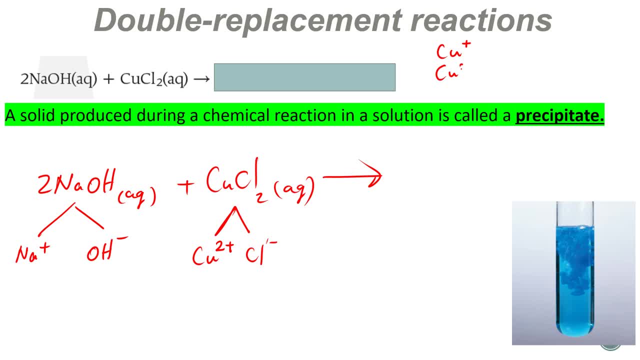 now Cu can be plus and can be plus 2, but because I have 2 here and we know that Cl minus 1 is charged, so of course the 2 comes from the plus 2. that's why the ion here is plus 2. so take this with this, take this with this, so you are going to get NaCl plus CuOH2. 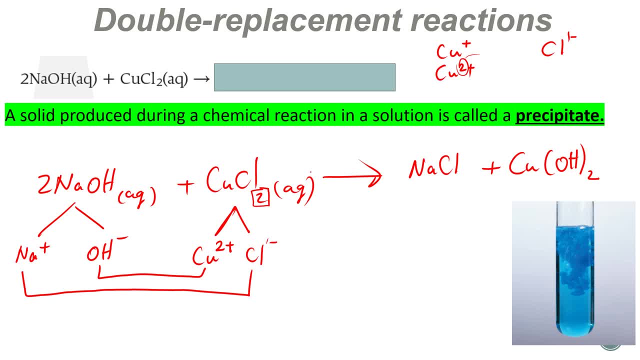 now balance the equation. okay, of course, this equation should be balanced already. I'll just have 2 here and that's it. so I'm trying to tell you here is that this compound, NaCl, is lukewarm water, but did you see these compounds that are being formed here? 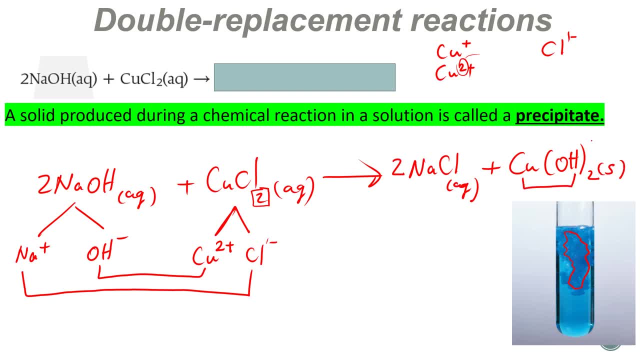 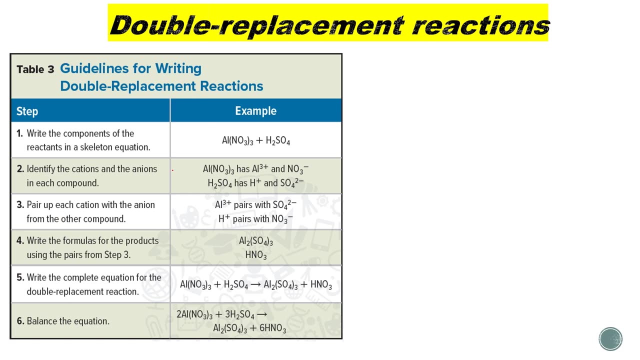 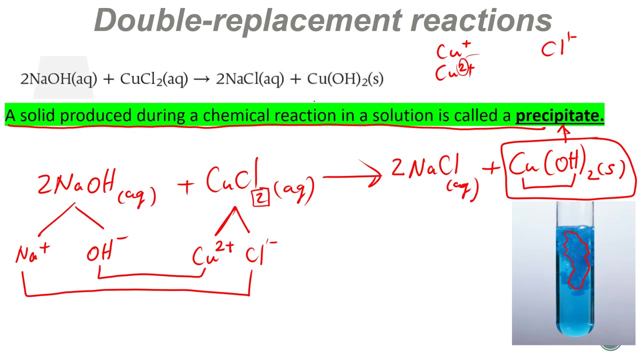 this is actually CuOH2. so what do we call this compound? we call it a precipitate. so a solid produced during a chemical reaction in a solution is called the precipitate. but what we applied here is this guideline and know how to do the double replacement reactions. okay, and as you. 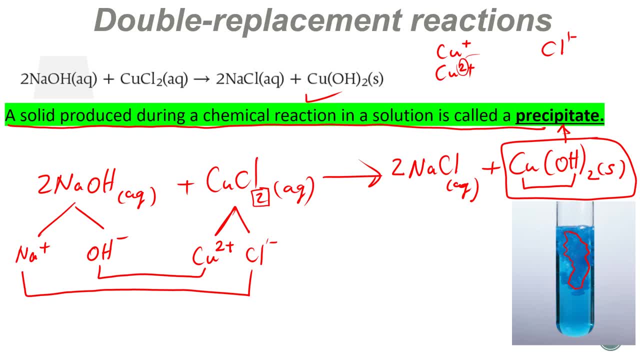 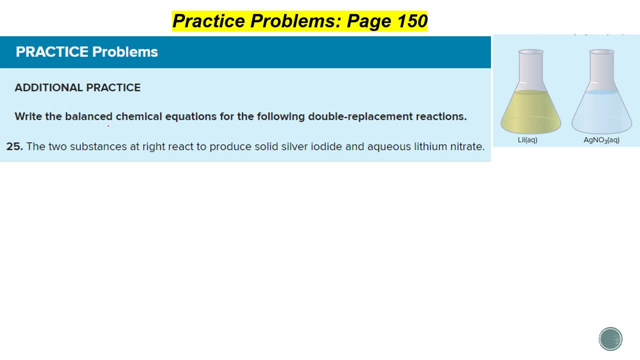 can see, this is the answer. so let's do this problem. guys. write the balanced chemical equations for the following double replacement reactions. so the two substances at right, elaalium, you need react to produce solid silver iodide and aqueous lithium nitrates. If we know how to convert the names into a form, we have to separate them into the first, very good, but I want to show you how we do it in here. so Li, so first thing, silver iodide, which is AGI, and lithium nitrate, which is LiNO3, but let's see how we can get this okay using what we actually learned. 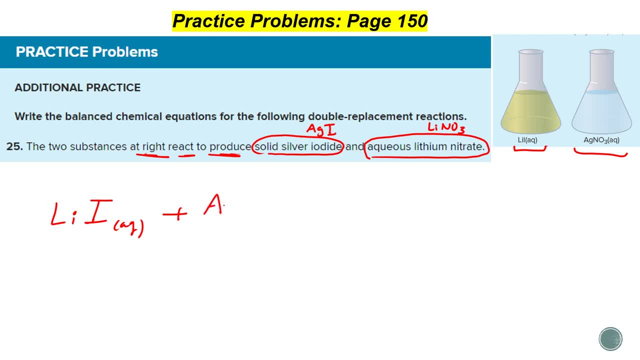 So AQ plus AGNO3, AQ gives me. so I told you first of all you need to find the ions in each one. so this is Li plus and this is I minus, because lithium is in group 1, and this is in group 17,. this is AG plus and this is NO3 minus. 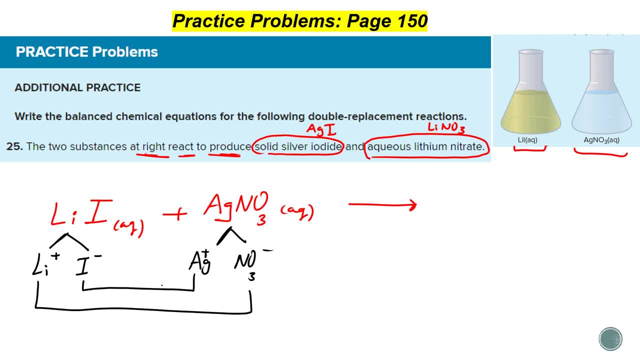 So positive with negative, Positive with negative. So here you get AGI and here you get LiNO3.. They are the two here, right? So you put AGI, they give you solid. so S plus LiNO3, AQ. 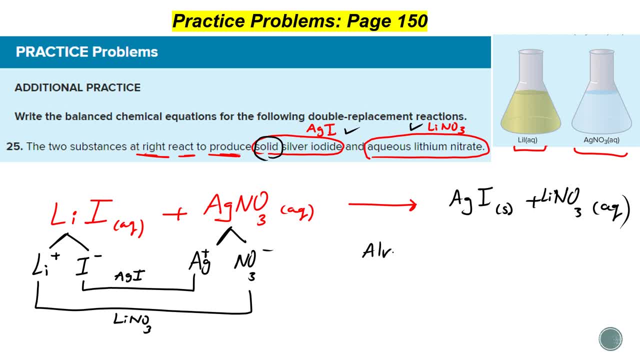 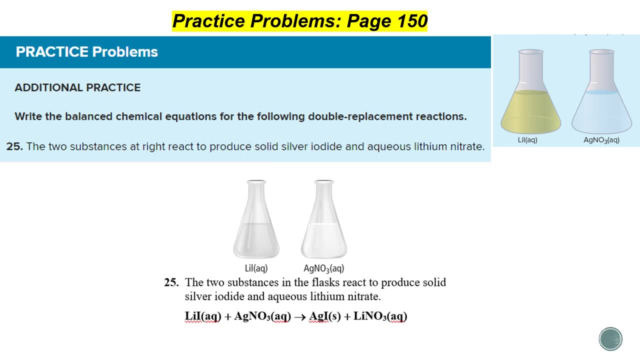 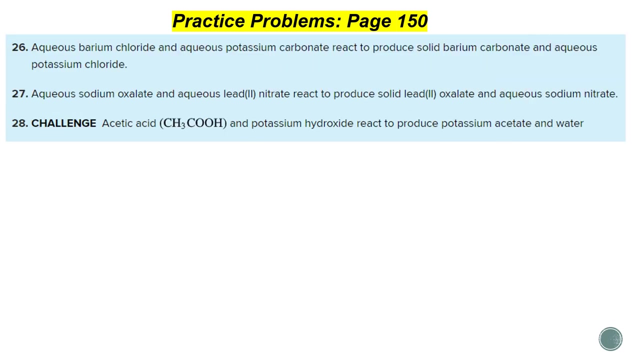 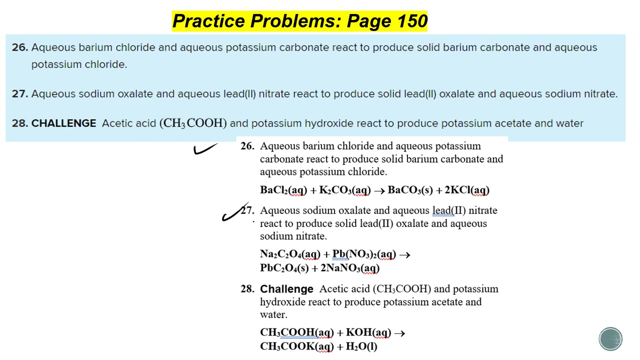 Do we need to balance anything here? No, this is already Balanced, Okay. So, as you can see down here, this is the answer. Now you have other problems here, okay, which you can try on your own. try to solve them on your own and you will find the solutions here for 26,, 27, and 28.. 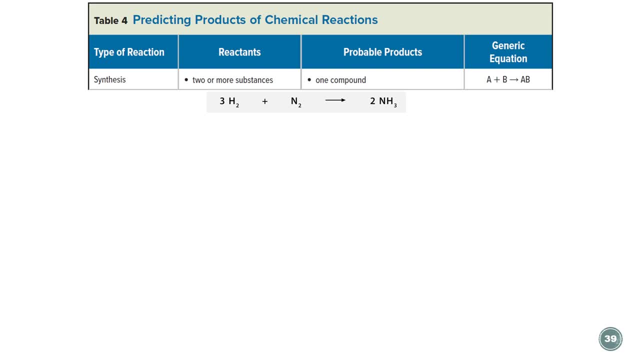 And that's the end of the lesson, guys. So we can now summarize what we have been talking about. We talked about synthesis reaction. We said that we have two or more reactants and one product, and this is the general formula. 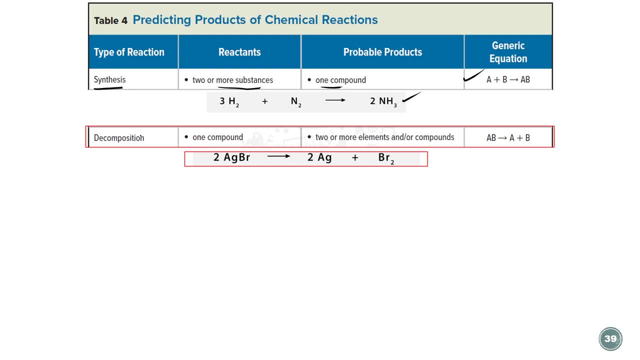 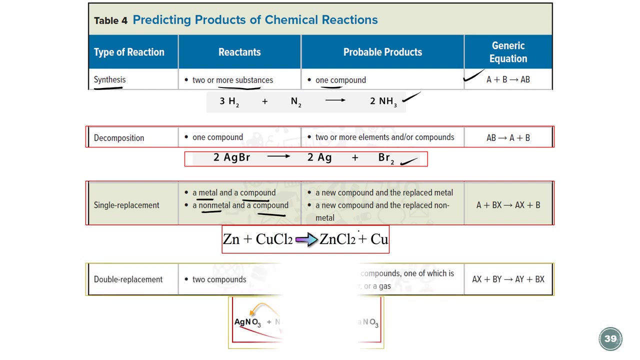 This is an example. We talked about decomposition reactions with this formula and this is an example. We talked about single replacement reactions, where it can be metal and the compound or non-metal, And we talked about double replacement reactions just right now. okay. 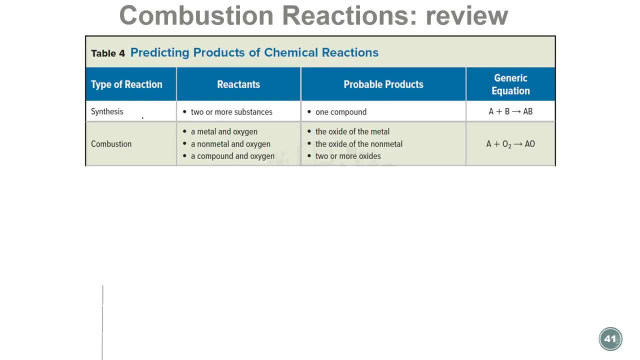 And sorry, and we talked about combustion reactions, okay, And the reactants can be metal with oxygen, non-metal with oxygen Compound with oxygen. The most important thing is that I have oxygen right, And this is the general formula, and this is just an example. 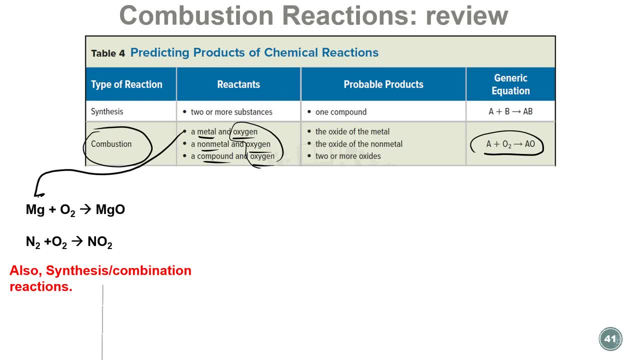 For example, this is a metal with oxygen. This is a non-metal with oxygen. Okay, So these are combustion reactions, And also synthesis. Okay, Now, this is here a compound with oxygen, Remember. So all of these are combustion reactions.